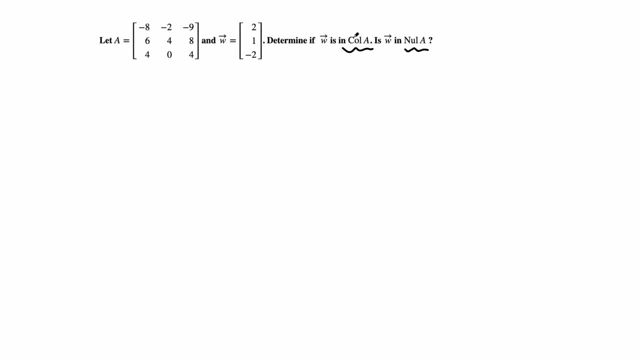 first let's do: if W is in column of A, So column of A, I mean. this question is in fact: is 2, 1 negative? 2 is a linear combination of these three column vectors and some constant times. the first one, So column of A, is negative 2 plus C2 times second plus C3 times third. Okay, let's say A1, A2, A3. 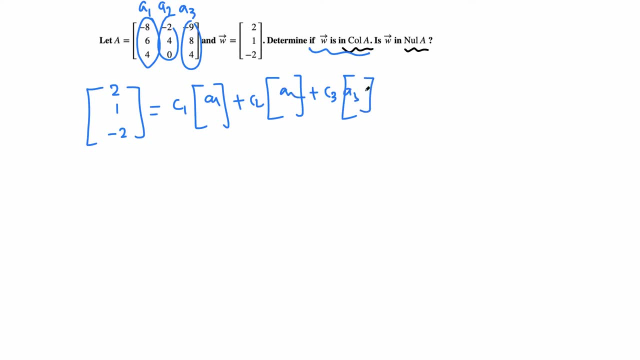 vector. they go here and is this true? So if we expand this, it comes out to be a system of three equations, and we know how to solve that. we can always turn that into an augmented matrix. So solving the solving, the solving. this is same as asking if the following augmented matrix, okay, is consistent. Let's see so. 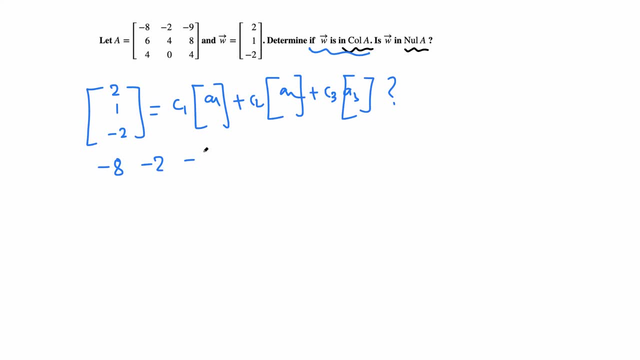 we write negative 8, negative 2, negative 9, 6, 4, 8, 4, 0, 4 and we got 2, 1, negative 2.. Okay so if we find the system consistent, then we are good. That means W is in column A If this system comes. 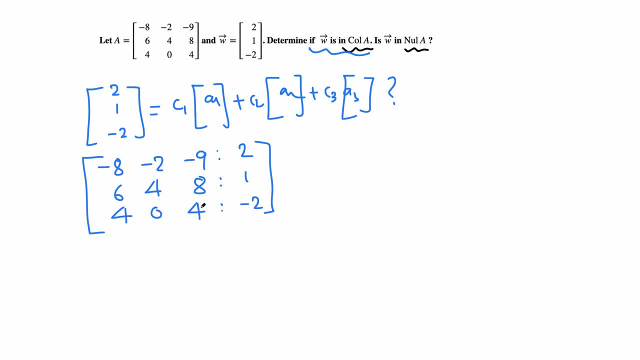 out to be inconsistent, like we got: 0 0 0 equals some number. that's inconsistent, okay, so let's do it. So we need to convert this into row echelon form. Try to make 1. that would be better, but here is a 4 0, 4.. 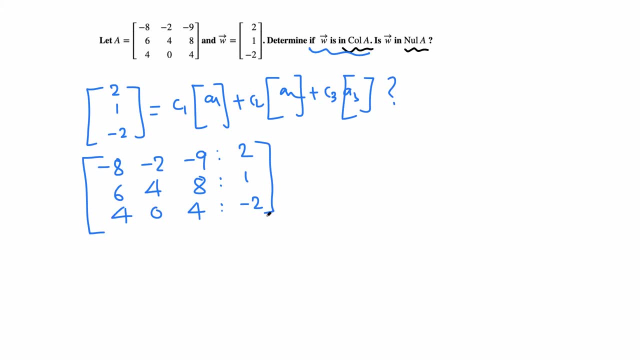 negative two. maybe interchange row one with row three. so row one and row three let's interchange. this is four zero four negative two. and here we got six, four eight. one negative eight, four negative eight negative two negative nine two. let's divide by multiply by one-fourth. so we're gonna work on r1 such that r1 is just 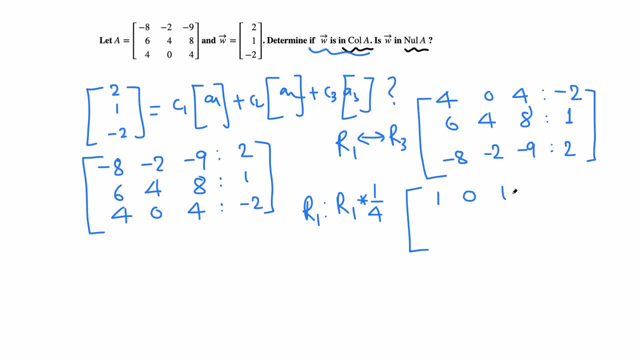 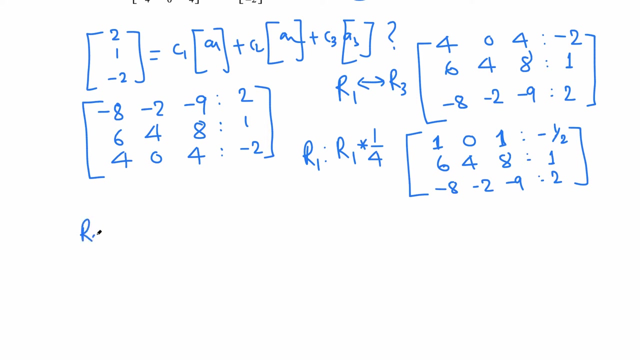 one-fourth. so this is one zero one negative one half. okay, now this is six, four, eight, one. here we go that negative eight negative two negative nine, two. okay, now let's make this zero, okay, this entry zero, using the very first entry, and also make this zero. so we're gonna work on two things here: r2, such that r2 plus. 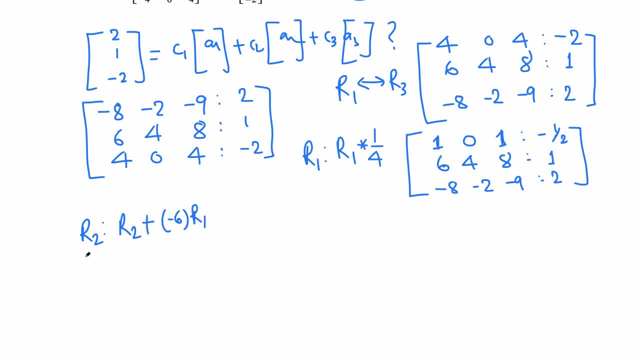 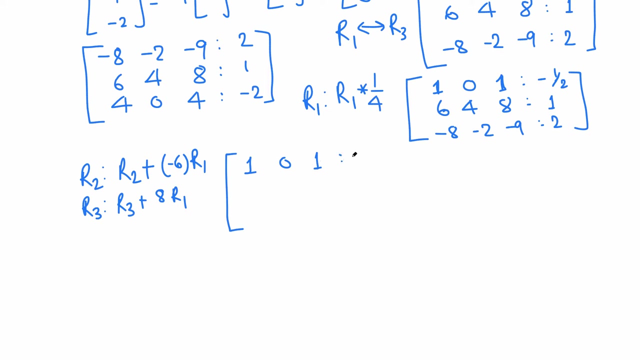 negative six times r1. okay, and at the same time r3 is negative eight. so plus eight times r1, so we are not doing anything on r1, so row one stays here. here now we are multiplying by negative six, so six negative six. zero, four, zero, zero. 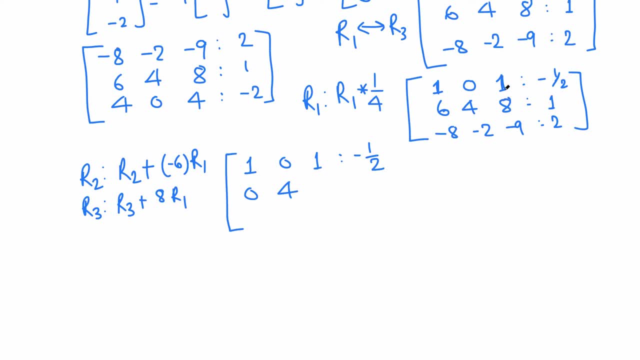 sorry, four, eight times negative. six, eight plus negative six, just two. one plus negative. six times negative. one half is three positive three. one plus three, it's gonna be four negative eight. we are multiplying by eight. negative eight plus eight: zero, just negative. two is eight. negative. nine plus eight is negative. 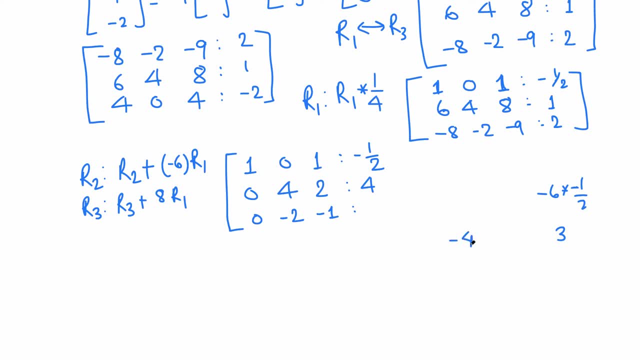 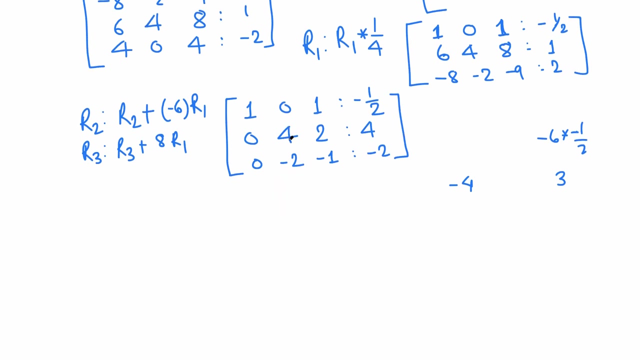 one, eight times negative. one half is negative four. so two plus negative four. two plus negative four is negative two. okay, now, next, we're gonna make this one so that we could make this zero, which is not necessary. uh, this is, we got pivot here. so let's make this zero, because four and two we can simply multiply. 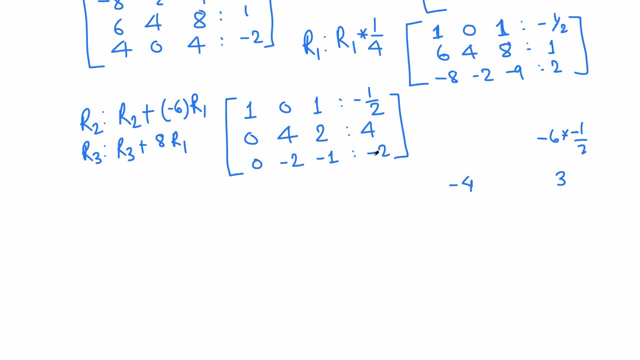 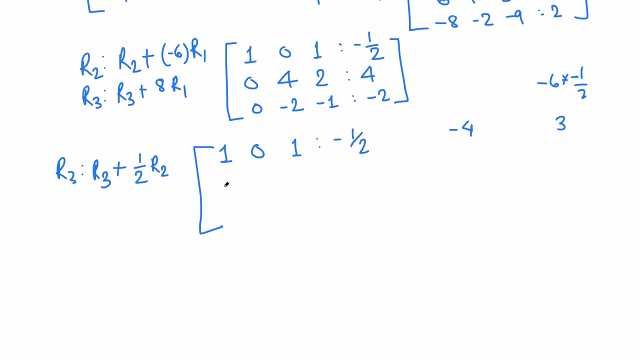 this by two and add, so we don't have to make this one, so still. or on r3, r3 plus, because negative two, so we can, in fact we can multiply by one half, because that's easy. one half, r2- okay, that makes we are not doing anything on r1: one zero, one negative. one half zero four, two, four. 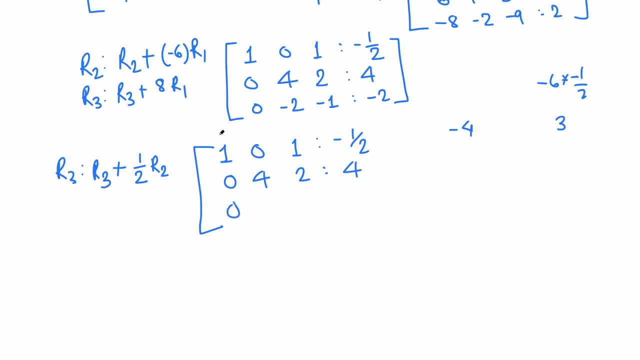 so zero, zero, zero. negative. two plus one half of four, that's positive. two. zero. negative. one plus one half of two, just one negative negative: one plus one half, that's zero. here we got negative two plus one half of r2, so that's also zero. oh, that's good. i mean consistent everything, zero. so we got a free variable here. 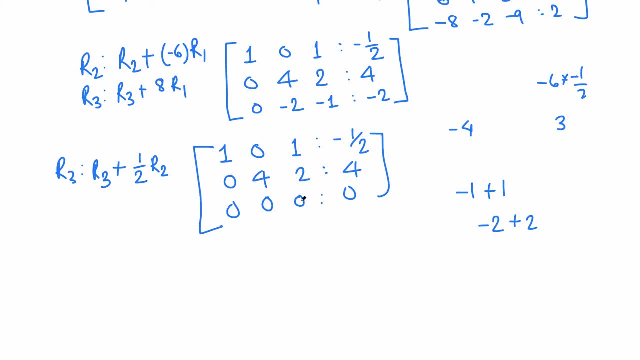 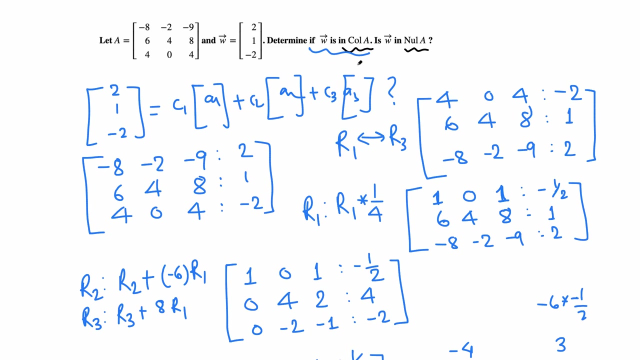 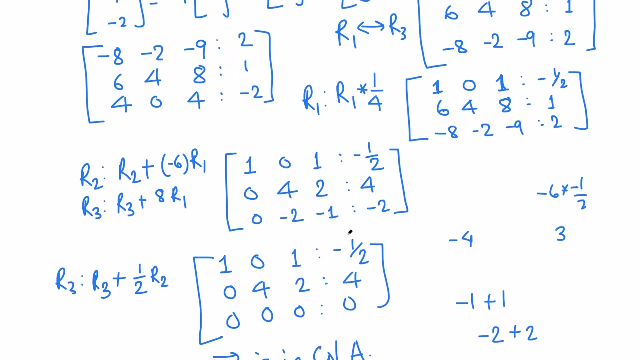 this is like c1, c2, c3 is free because there is no pivot here, but the system is consistent. okay, this implies: yes, w is in the null, sorry, is in column of a, is in column space of a because a linear combination of these three columns, these three column vectors, 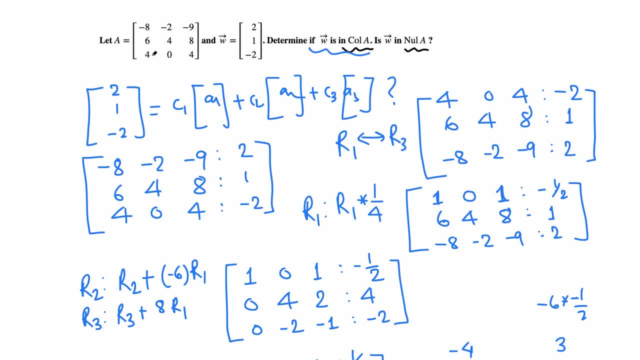 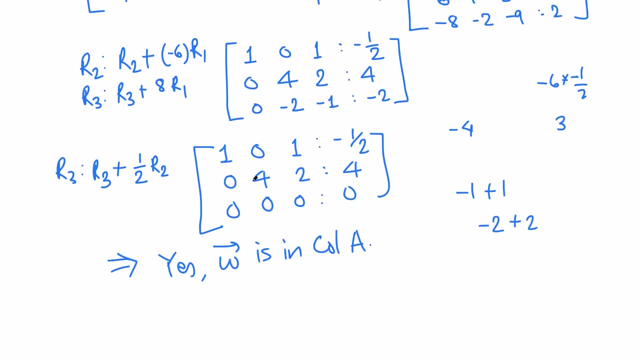 okay, the linear combination of this. in fact, since we found a free variable there, you can easily see this will be in a linear combination of these three. okay, in fact, if the question asks you to find the exact linear combination, you can solve for c1, c2, c3, because c3 is free. then you find c2 using this equation and c1 using this. 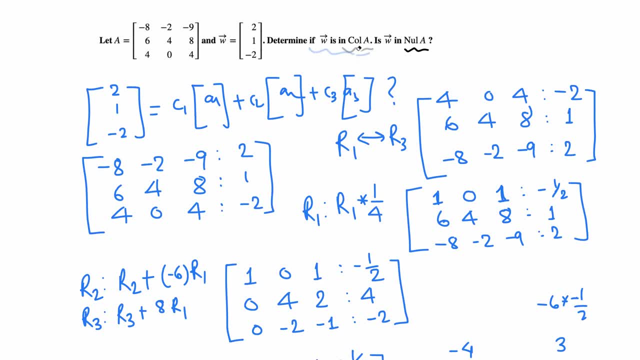 okay, so we just saw that this one is yes. now is w in null of a null space means all the column vectors that are mapped to zero. so we simply multiply this to a, w, a to w if it is zero vector. if it goes to zero, that means w is in. 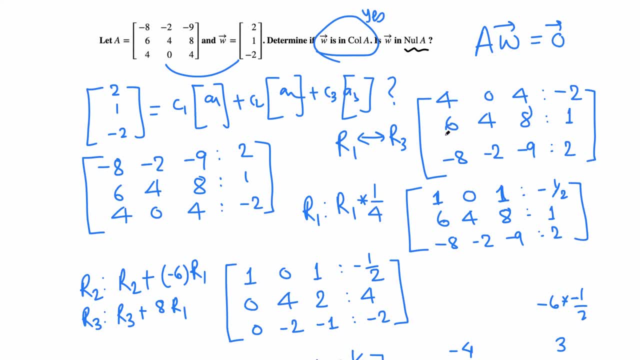 null space of a. so it's pretty simple. so let's just multiply here, and this should be done in here. so aw is, i'm answering the second part, negative eight. in fact. i don't have to even write here, let me just multiply. so this was what i was going to write. so i am going to write here. so